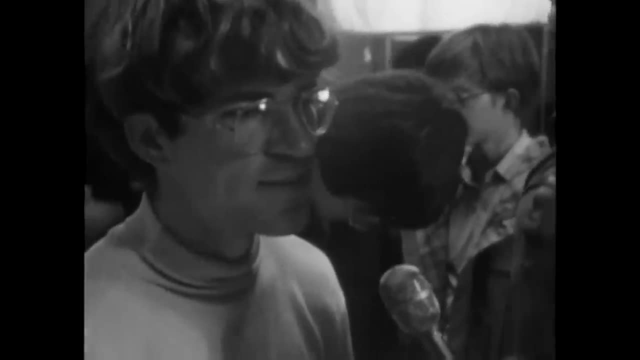 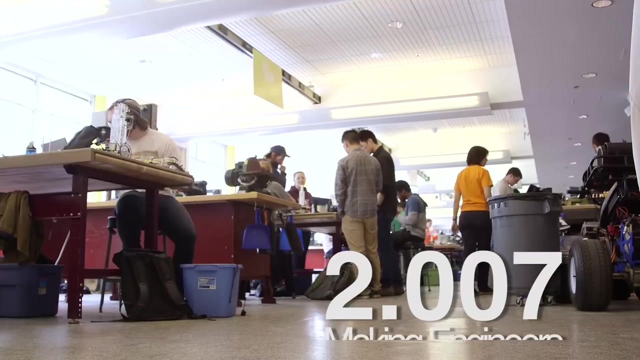 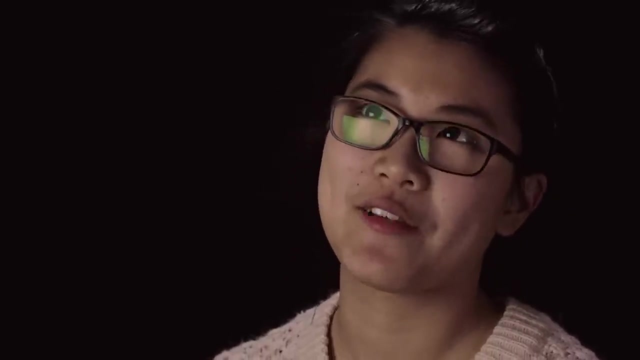 and the ideas over here were really incredible. The real innovation was to build a device and make sure that you not only designed it, but you built it. It's the class I've been waiting for. I think it's the class that every mechanical engineering. 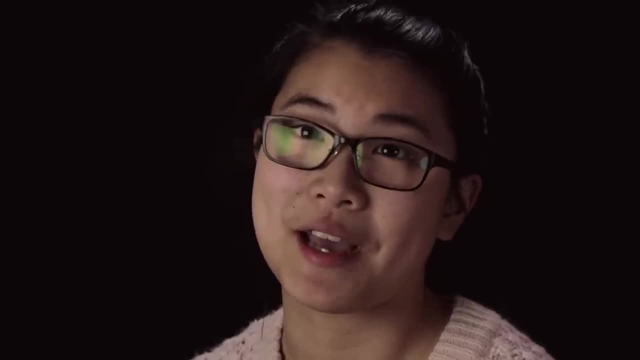 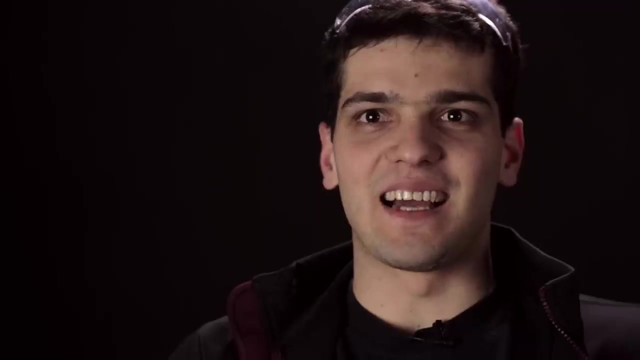 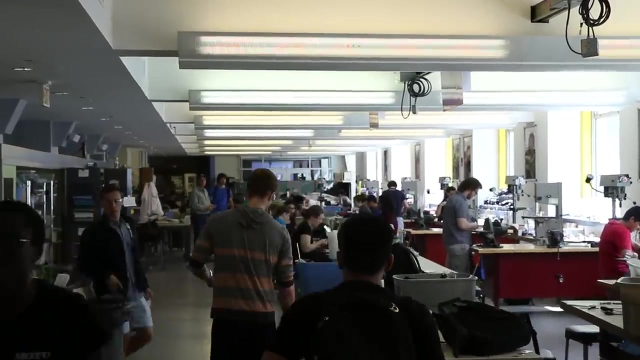 major wants to do as soon as they declare mechanical engineering. The reason why I chose mechanical engineering is because I like making things. This is the class where you make things. This is what I went to MIT for. It's the first time MechE students at MIT are coming in. 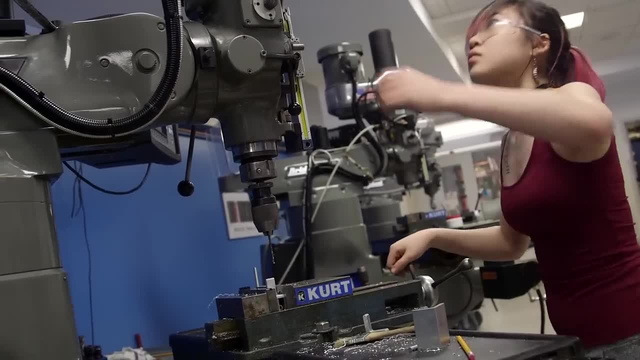 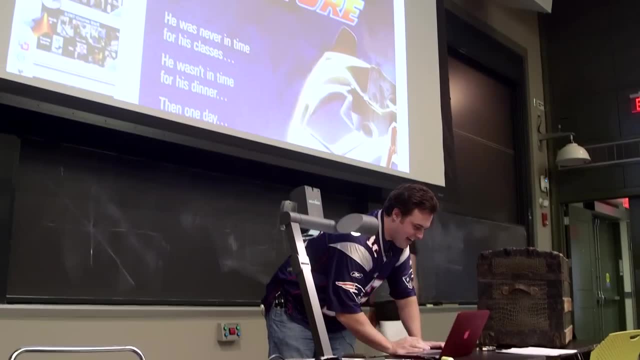 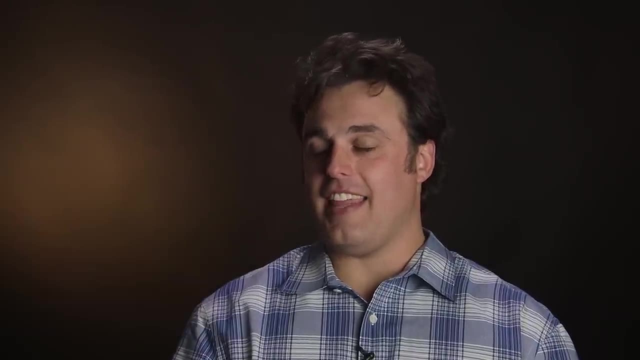 They're in contact with the big machines and the workshop, And this is really the class where you take everything that you've learned in those lecture halls and you put it to use. Okay, it is time to design. When I took 007 over, I was very honored because this is a historic class and I think it embodies 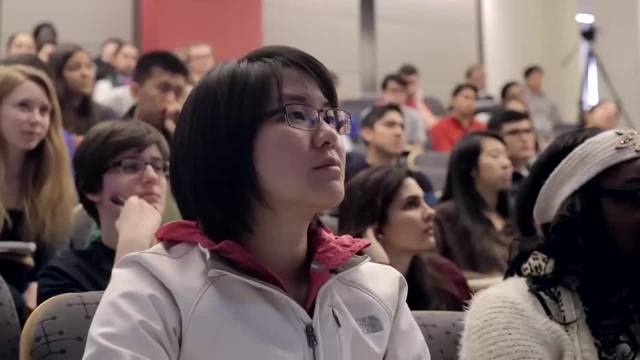 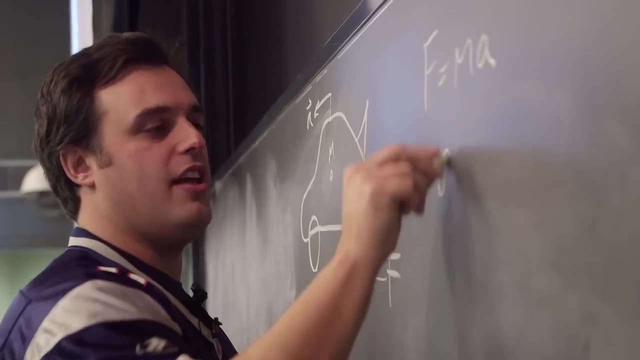 the spirit of MIT. It's the first experience students have designing something on their own. I'm starting to see how what I'm learning applies to the real world. This is the first time MechE students have designed something on their own. I'm starting. 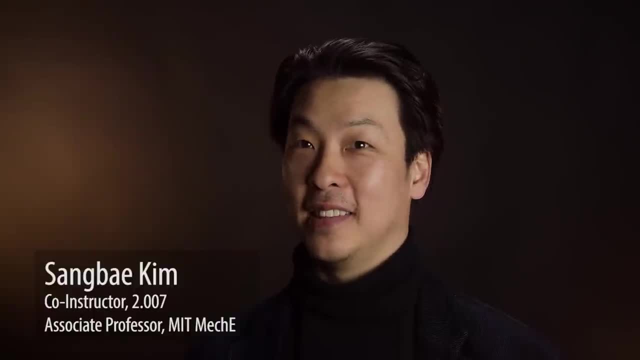 to see how what I'm learning applies to the real world. This is the first time MechE students have designed something on their own. I'm starting to see how what I'm learning applies to the real world. This is the first time MechE students have designed something on their own. I'm starting 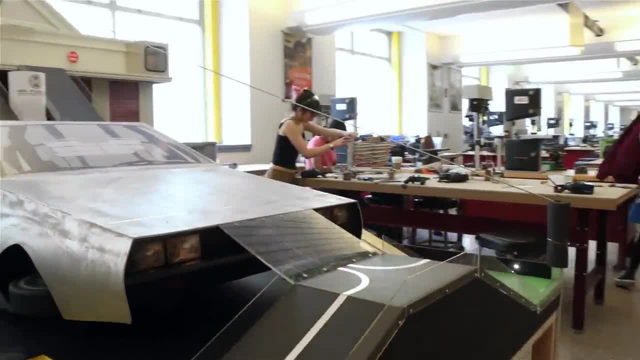 to see how what I'm learning applies to the real world. I'm starting to see how what class represents the MIT's model mind and hand exactly. So the theme this year is Hack to the Future, which features a giant DeLorean on the game. 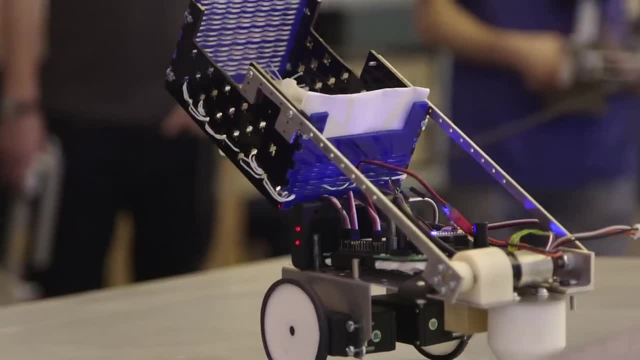 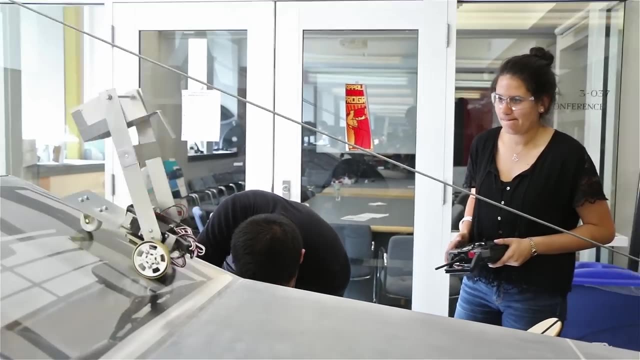 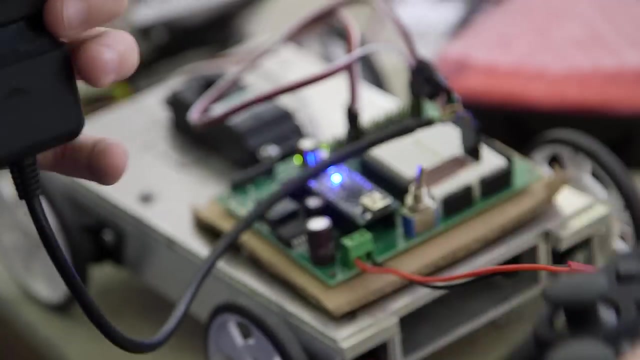 board. We build the competition around good mechanical engineering principles like climbing hills, optimizing power, managing friction, but all the time mix in cutting-edge new engineering innovations. Now it's chips and electronics as well as mech. Now it's chips and electronics as well as mech. 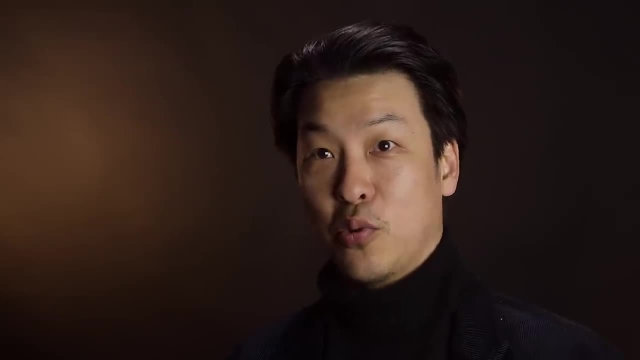 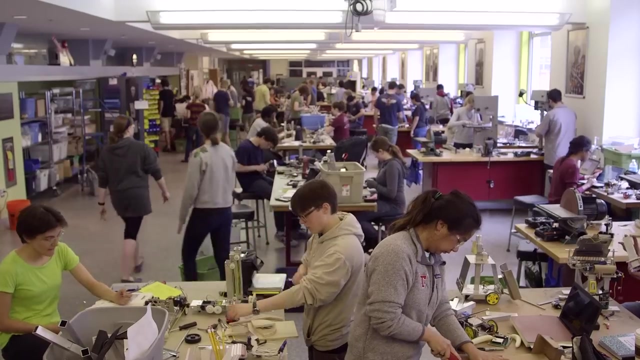 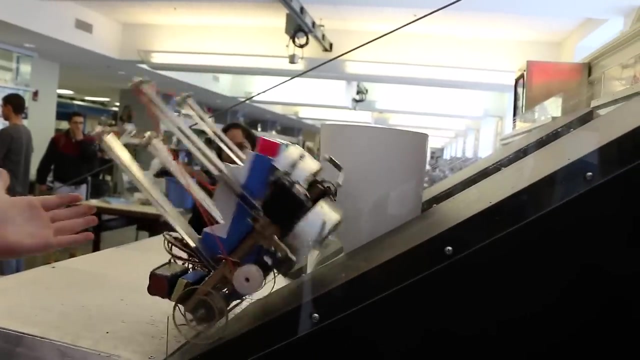 well as things like 3D printing. They actually get to program the robot using microprocessors. It's what the world is doing right now. This is such a real life experience for the students. They're making something that works perfectly on paper and then performs terribly in real life, And that's what happens to all of.